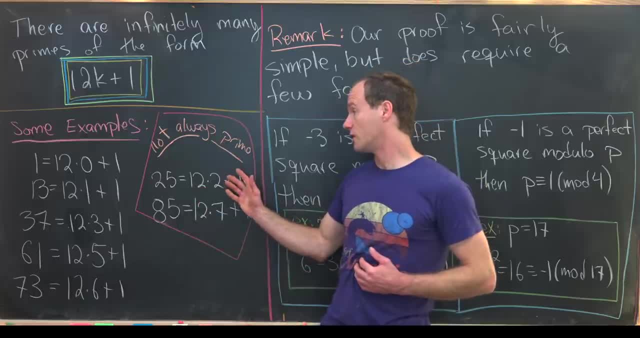 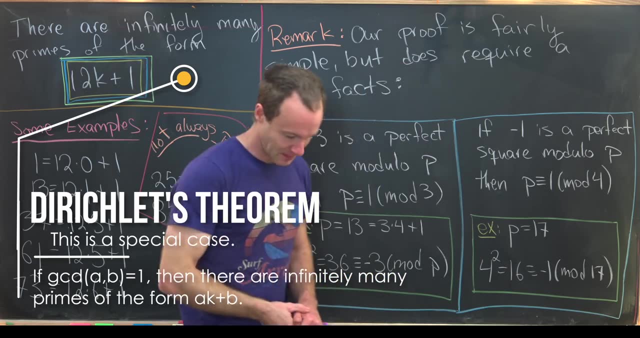 there's some in between there as well. So, even though not all of them are prime, there are in fact infinitely many primes on the list of numbers of this form, And that's what we're going to prove today. And before we get started, I want to make a remark, And that is our proof is fairly simple. 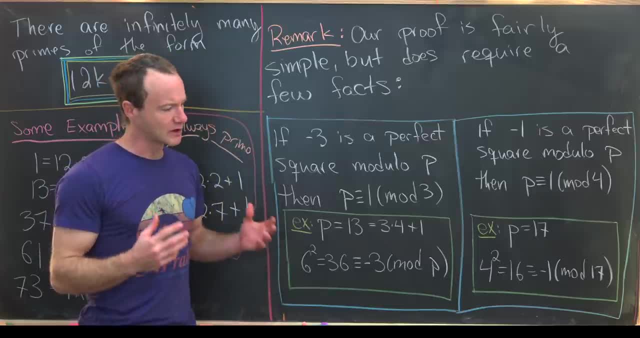 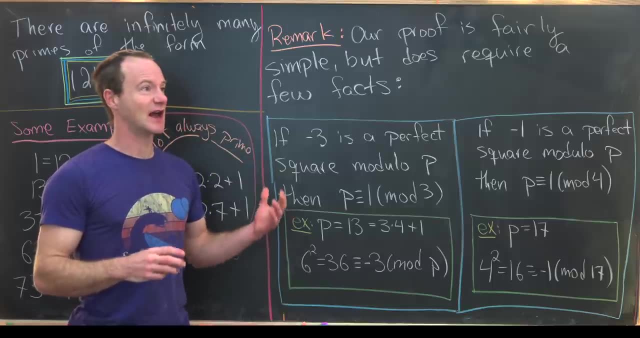 but it does require a few facts. And if you're more interested in understanding these facts more closely, I want to make a remark, And that is our proof is fairly simple, but it does require more deeply. I urge you guys to check out my elementary number theory course I've got. 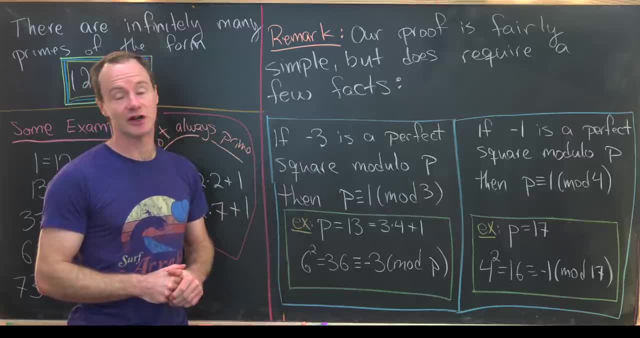 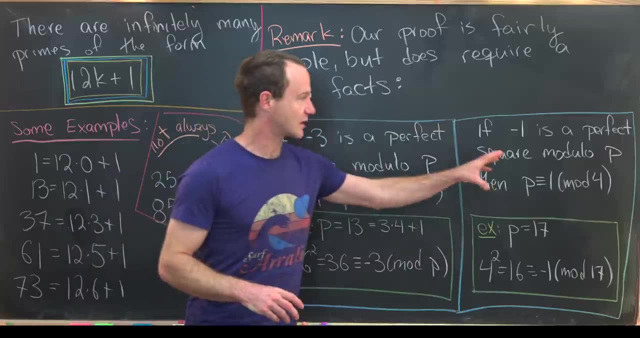 actually two versions of it: One like older version when I just started YouTube, and one newer version, which I'm still uploading videos to right now. Okay, The two facts that we're going to use have to do with when something is a perfect square, And this would be categorized under the 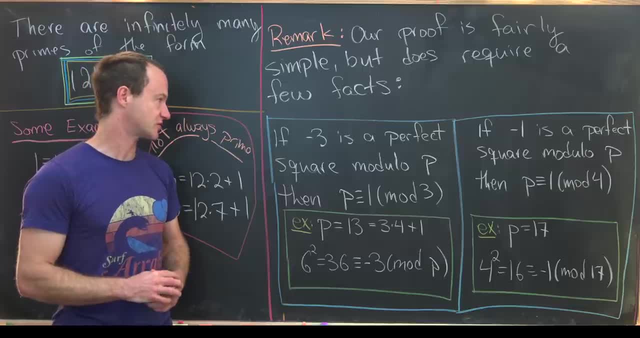 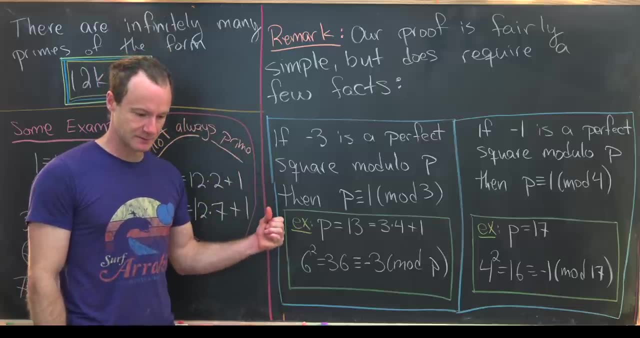 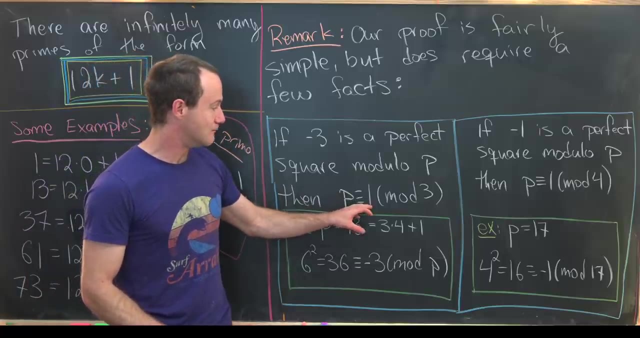 notion of quadratic residues, if you want a keyword to search. So if minus three is a perfect square modulo p, in other words we've got a prime and mod that prime negative three happens to be a perfect square, Well then that means this prime must be one mod three. It's impossible for this. 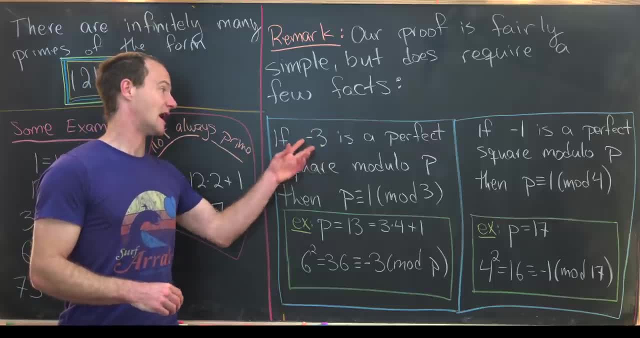 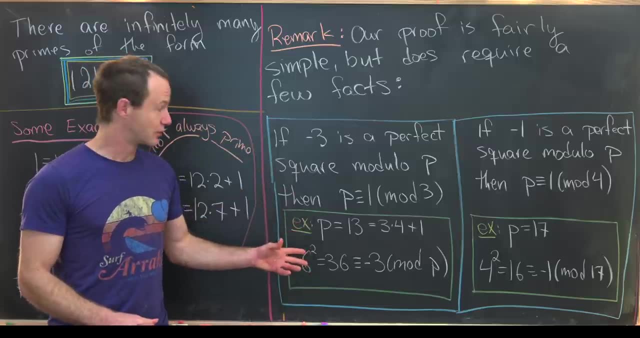 prime to be equal to two mod three and allow minus three to be a perfect square. So let's just see an example of that happening real quick. This is obviously not a proof of this situation. A proof of this situation would be found either in a homework to the computer or in a homework to the 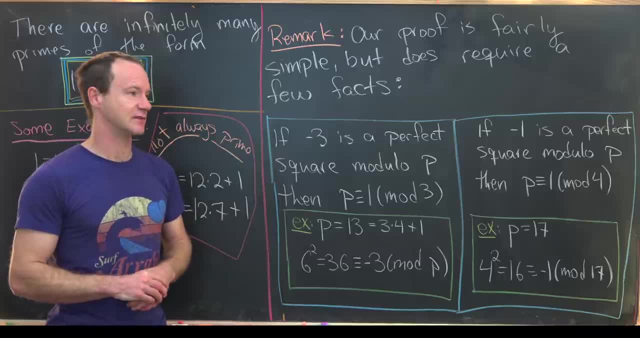 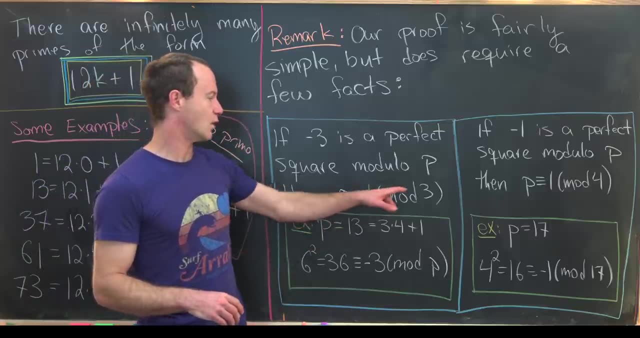 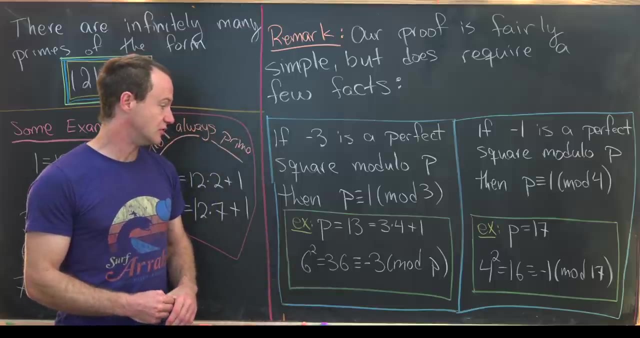 course that I am giving, or in a lecture for the course that I'm giving. Some of these are in the videos that I've done. Okay, So if p is equal to 13,, so notice, that's most definitely one mod three, It's three times four plus one. Then negative three is equal to 10 in this case. Well, that's. 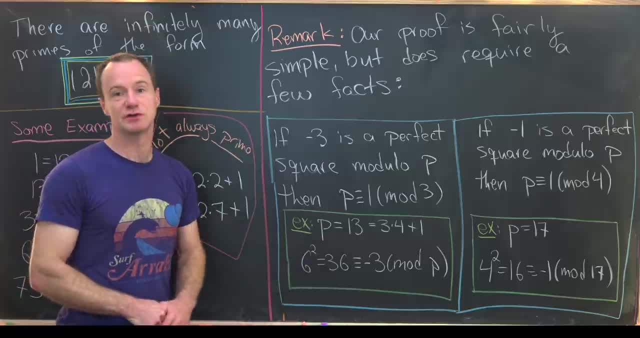 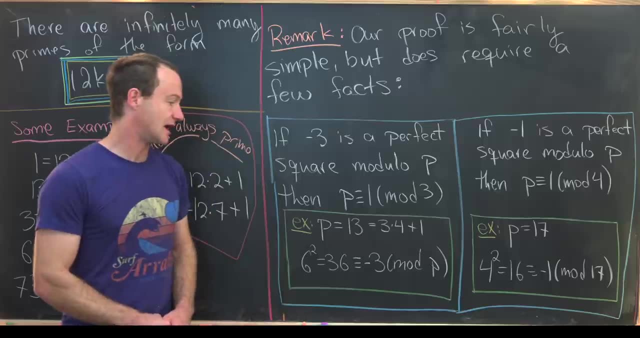 pretty clear, because we're 13,. but notice: six squared is equal to 36.. 36 is 10 more than 26,, which means it's negative three mod our prime, which is 13 in this case. Then the other fact that we'll use is: 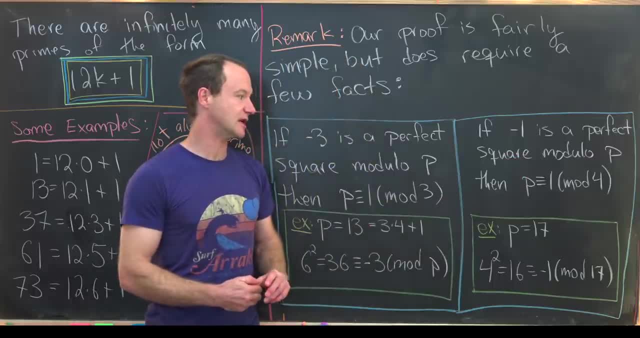 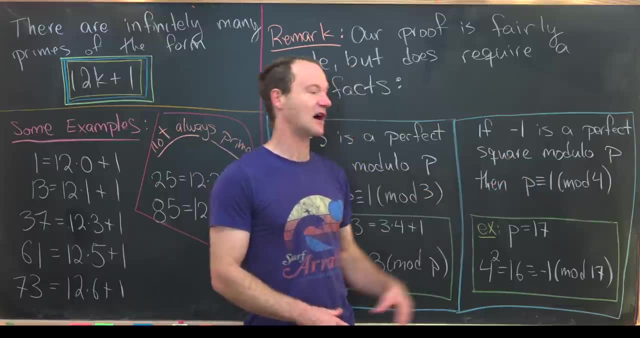 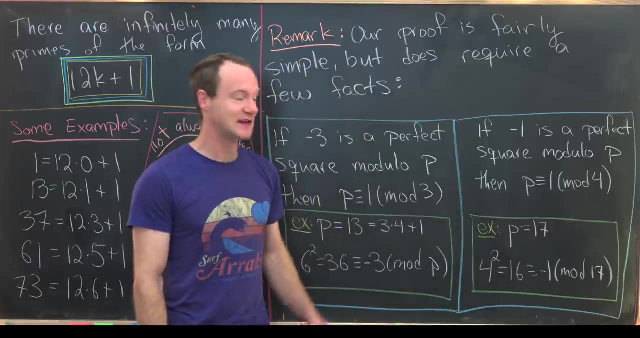 negative one is a perfect square, modulo p, if, and only if, p is congruent to one mod four. So those are the only types of primes that allow for minus one to be a perfect square. Let's look at a quick example of that. So p equals 17.. That's obviously one mod four. It's four times four plus one. 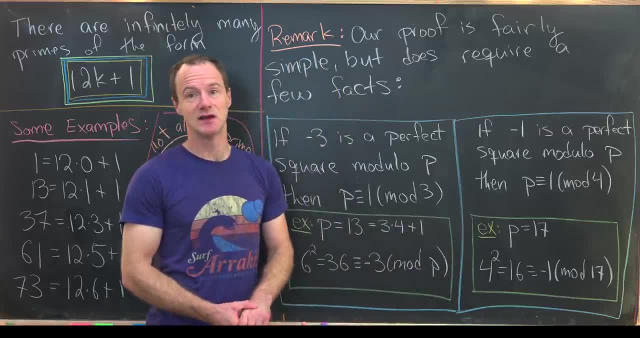 And then if we look at a perfect square, it's one mod four. So that's obviously one mod four. So if we look at four squared, we get 16, but 16 is one less than 17,, which means it's minus one mod. 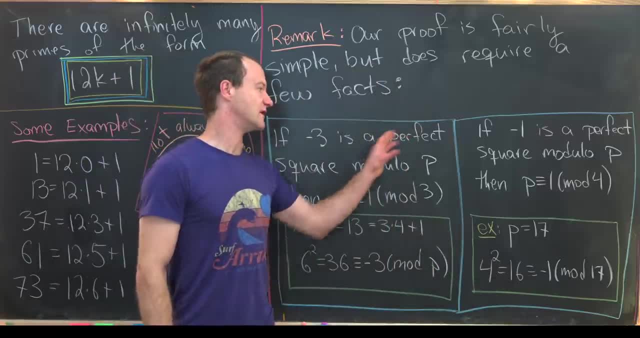 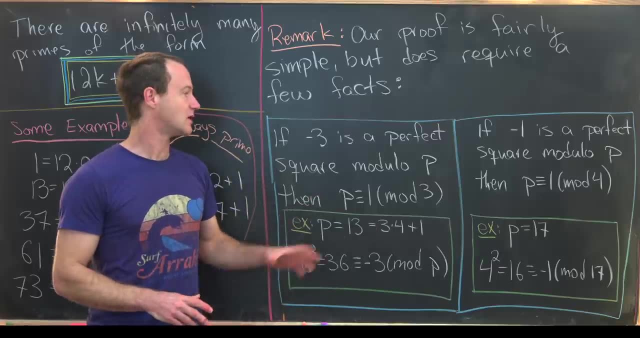 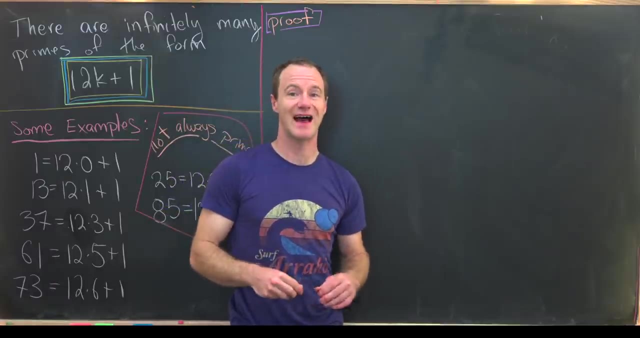 17. So there's a situation showing that these two facts are true, at least in these cases. Okay, So now that we've set up the problem, along with facts that we'll use, let's dive into the proof. Okay, Now that we've provided some background along with a couple of facts, 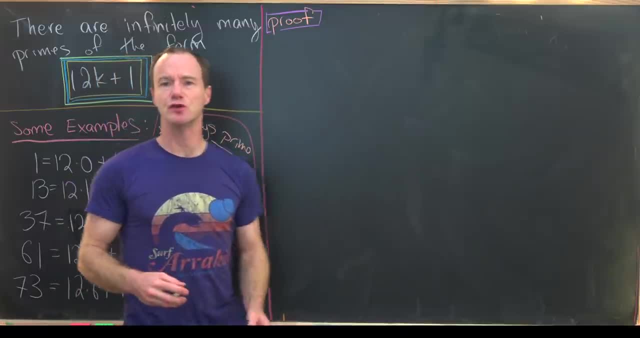 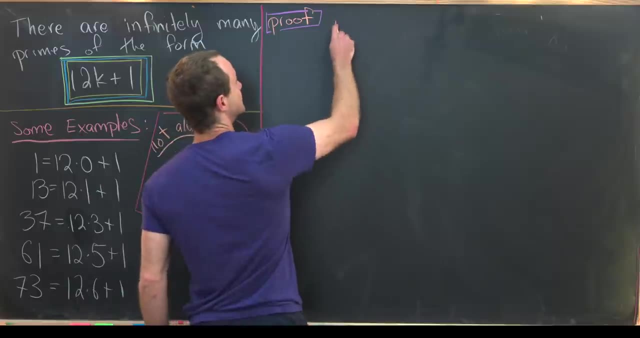 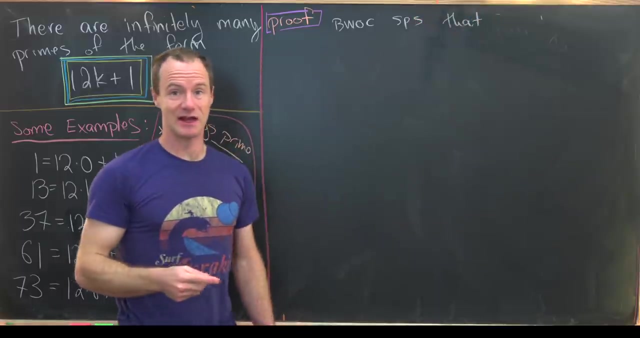 let's jump into the proof, And so, just like we do with a lot of different, infinitely many primes of the form type proofs, we're going to do this by way of contradiction. So let's, by way of contradiction, suppose that there are only finitely many primes of this form. 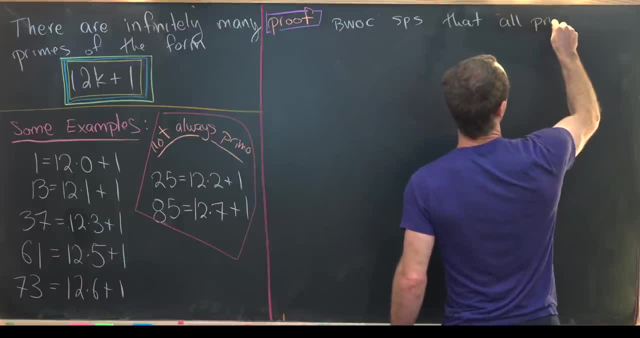 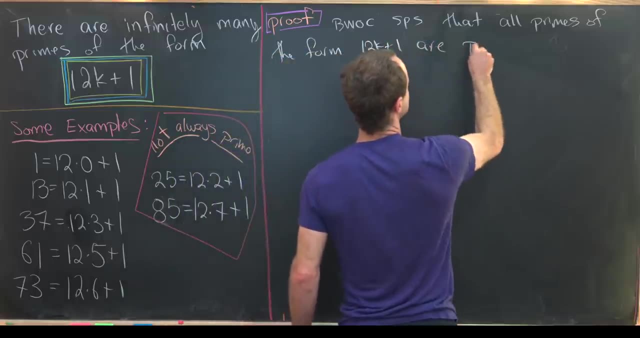 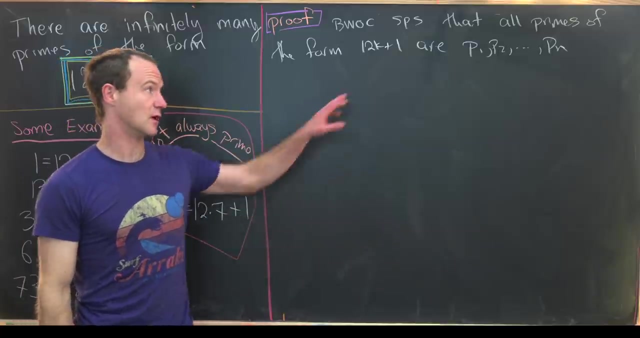 So we can write that as follows: that all primes of the form 12k plus one are on this list: p1, p2, up to pn. So there are only n primes of this form. Well, that's finitely many. Okay, great. And now we want to set a number, which I'll 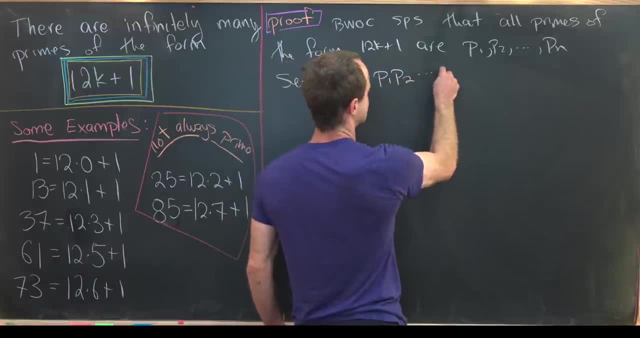 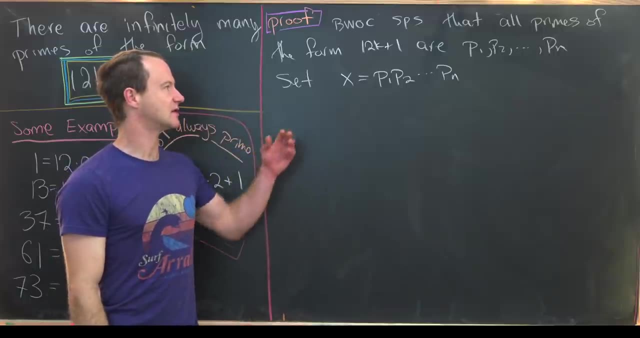 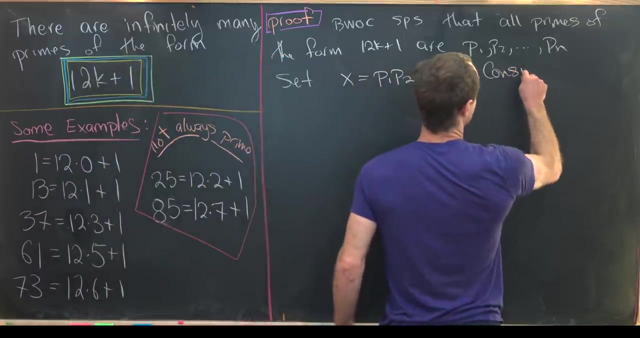 call x equal to the product of all of these. So these are standard first steps for primes of the form proofs. Now we're going to consider a polynomial built out of x and we'll give that a name n, So let's maybe write that down. So we're going to consider the following number: 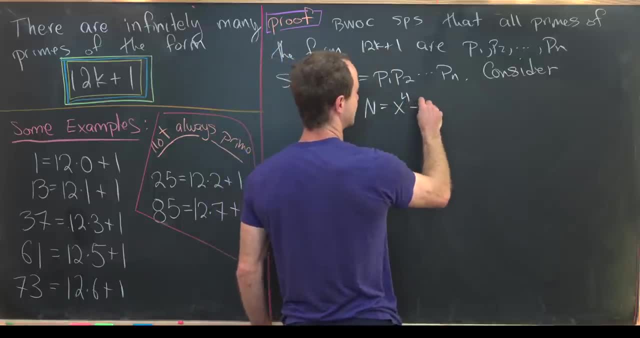 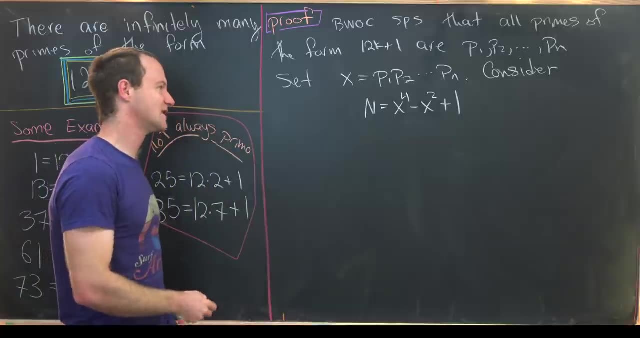 I said we'll call it n, So that'll. this will be x to the fourth minus x, squared plus one. that seems like it might have come out of nowhere, But this will actually be really helpful. So next, since this is a natural number, 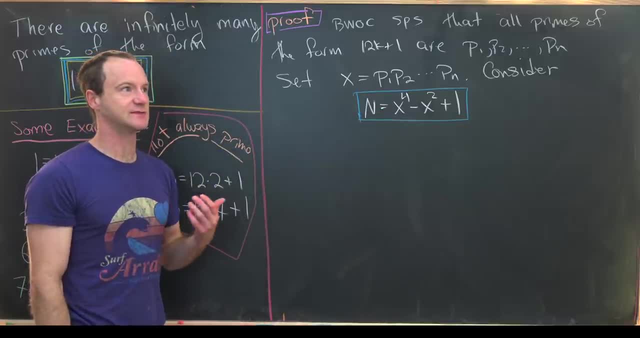 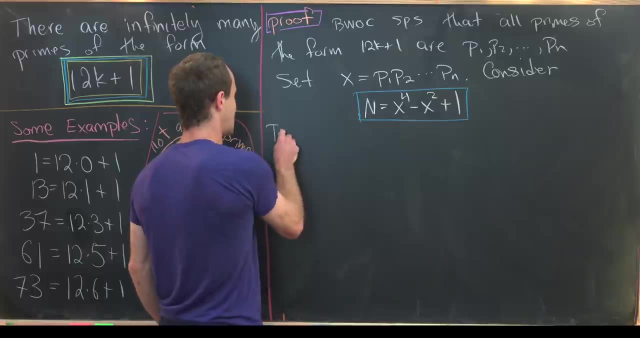 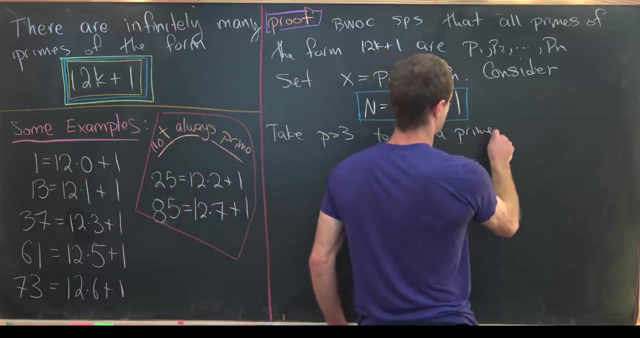 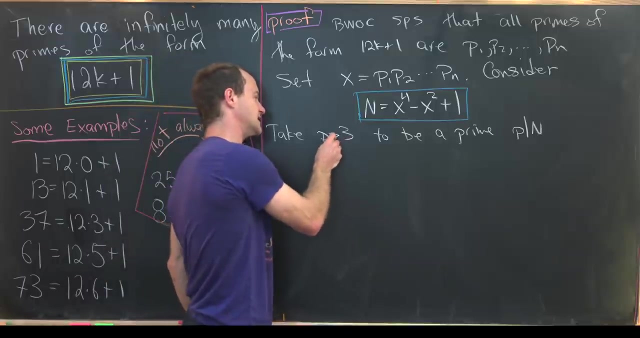 it has a prime divisor. We know that because by the fundamental theorem of arithmetic, every natural number can be factored into primes. So now let's take p bigger than three to be a prime, Such that p divides n. So I'll let you guys think about why we're able to pick this p to. 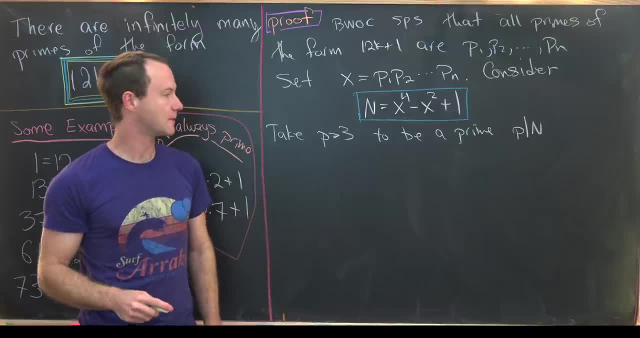 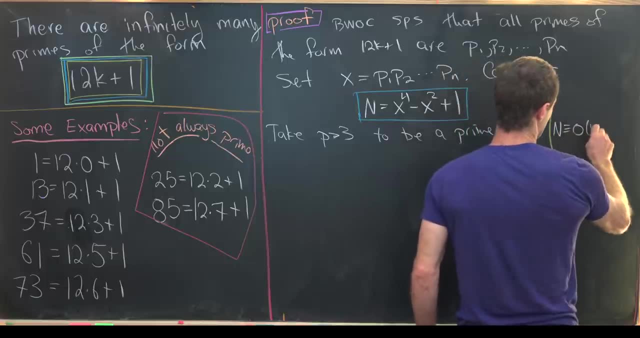 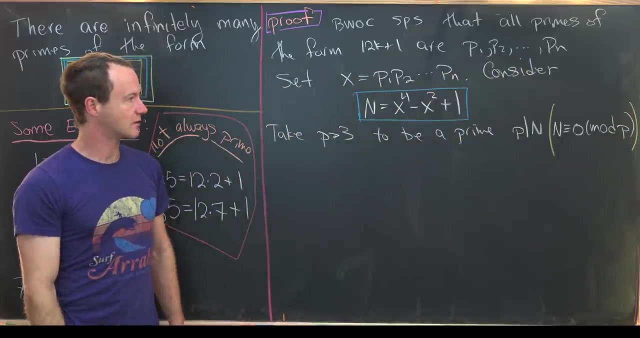 be bigger than three, But that shouldn't be too hard to think about. Okay, but notice, if p divides n, that's the same thing as n is congruent to zero mod p using the notion of congruence modulo p. Okay, so where can we go from here? So now I'm going to replace n with this polynomial thing. 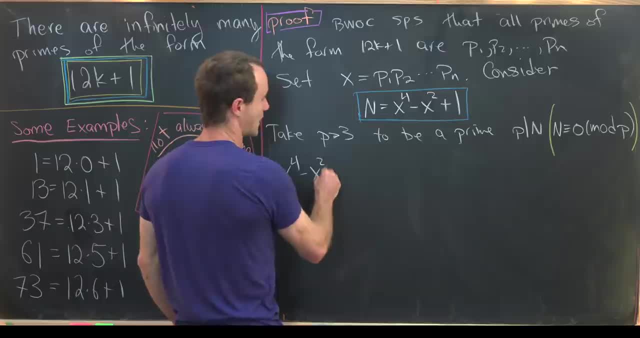 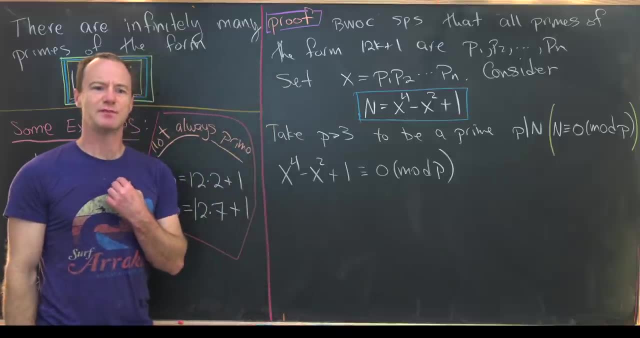 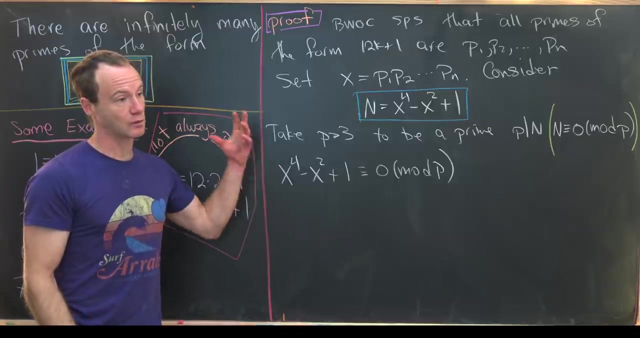 so we've got x to the fourth minus x. squared plus one, is congruent to zero modulo p. Now we want to build this into a perfect square two different ways, with two different numbers on the right hand side, And then that will restrict the values of p that are possible. And then we can. 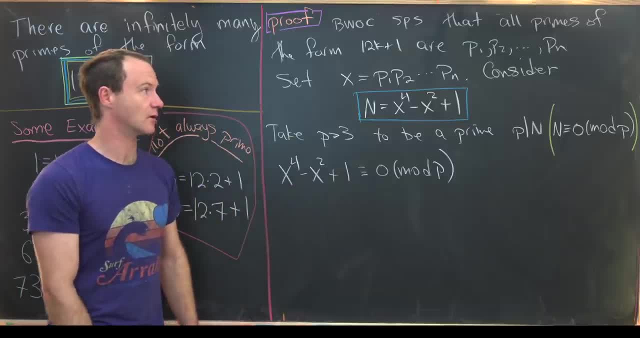 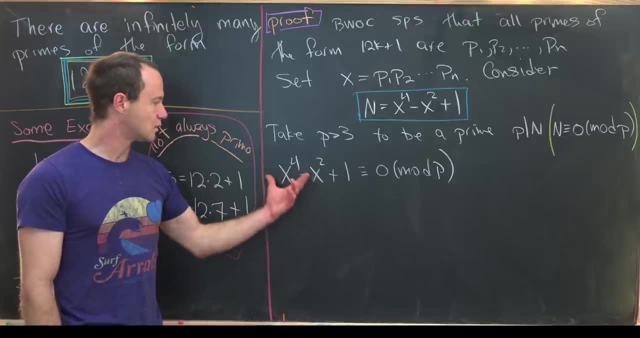 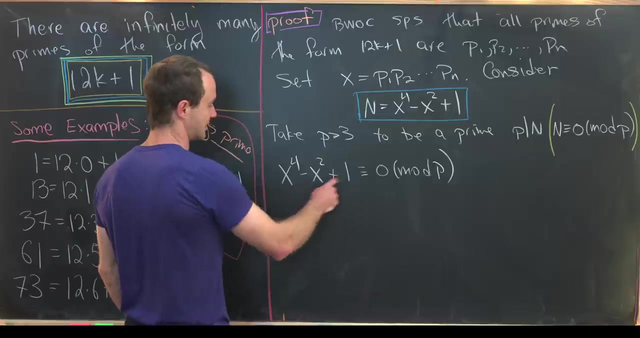 glue those together to show that p has to be a certain form. And in fact we'll show that it has to be a certain form. So we'll start by completing the square with parts of this object. So we can do that by first multiplying this whole thing by four. that'll give us four x to the fourth minus. 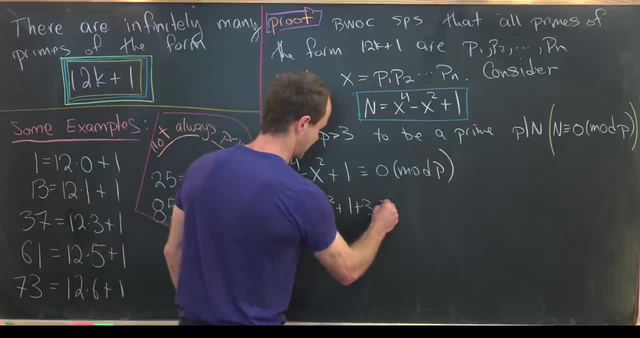 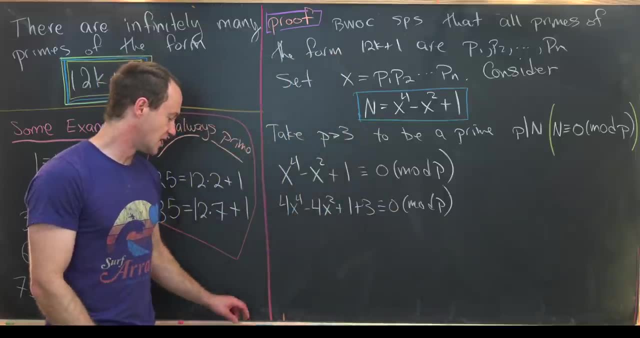 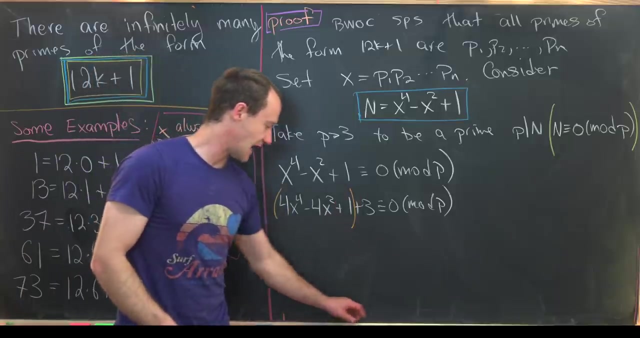 four x squared plus one plus three, congruent to negative, congruent to zero mod p. So I've split the plus four into plus one plus three, And that's because now I can take this stuff, which is an orange, and write it as a perfect square binomial, And then I can take this three and move it over to 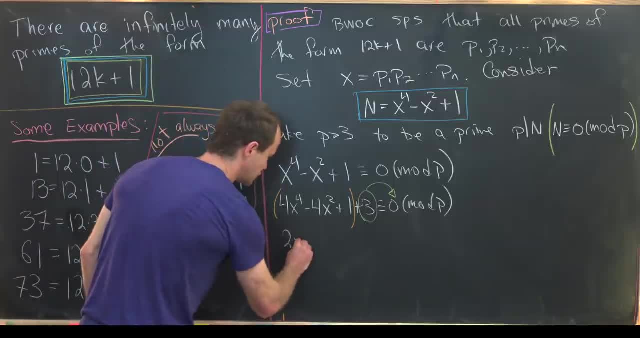 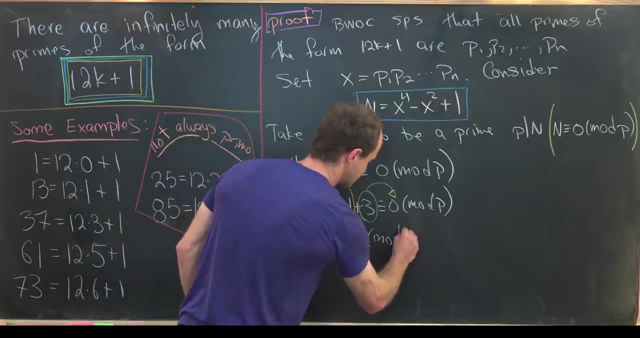 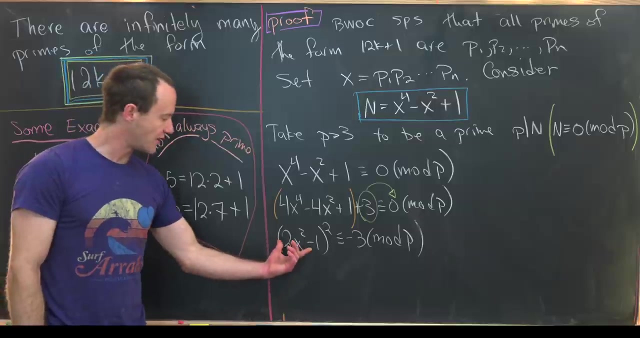 the other side of the congruence. So that's going to give us two x squared minus one squared, congruent to negative three modulo p. But it doesn't really matter that we have two x squared minus one over here. All that matters is that we have a perfect square on the left hand side. 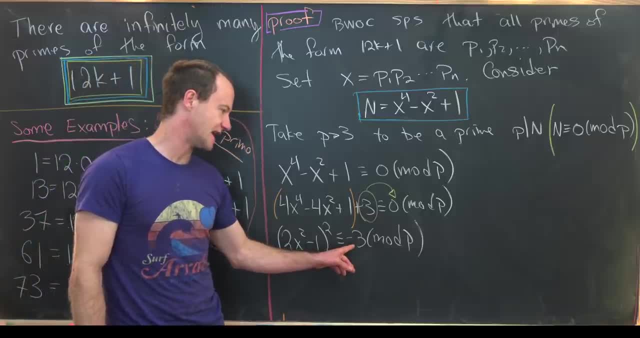 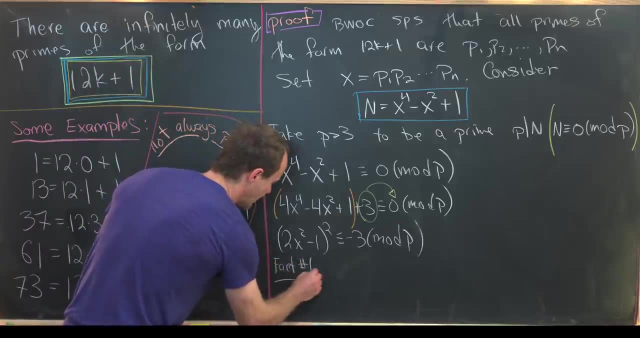 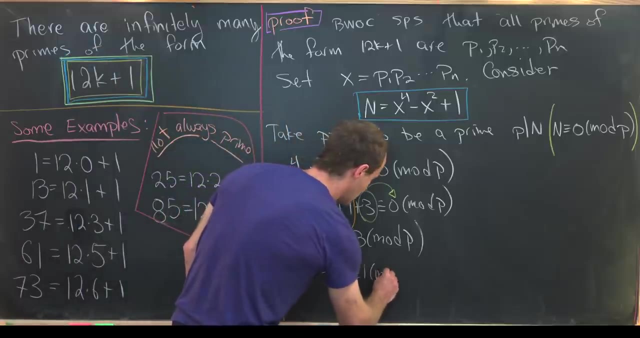 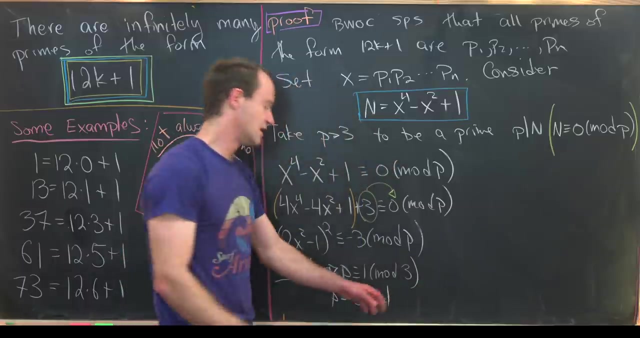 So we have a perfect square- is congruent to negative three mod p. But then by our first fact- so I'll call it fact number one- that tells us the form of p. So that means p is congruent to one modulo three. In other words, p is equal to three m plus one for some value of m. So that's an. 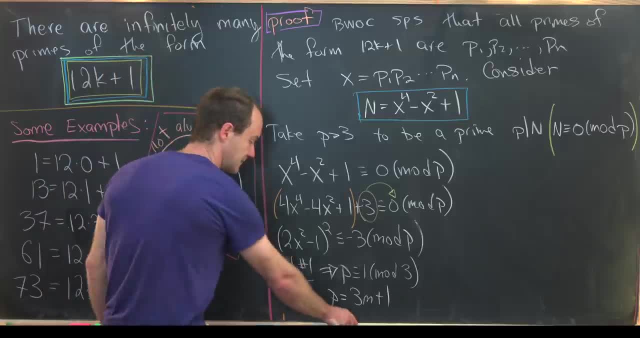 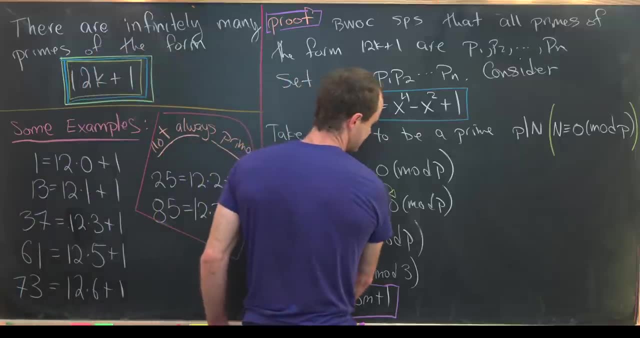 equivalent definition of being congruent to one mod, p. So we have a perfect square: is congruent to p. okay, so let's maybe square this in purple and then we'll move on to the next bit of this. now we're going to take this congruence, rewrite it and then do a little linear combination with. 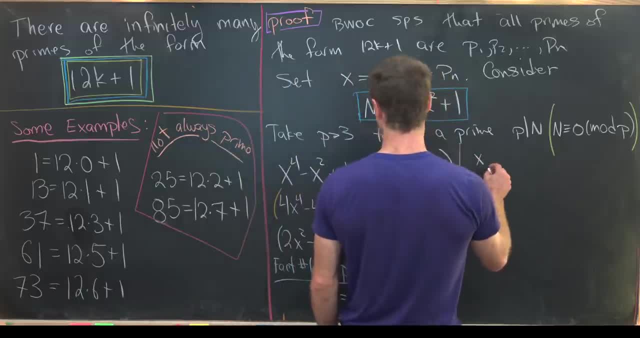 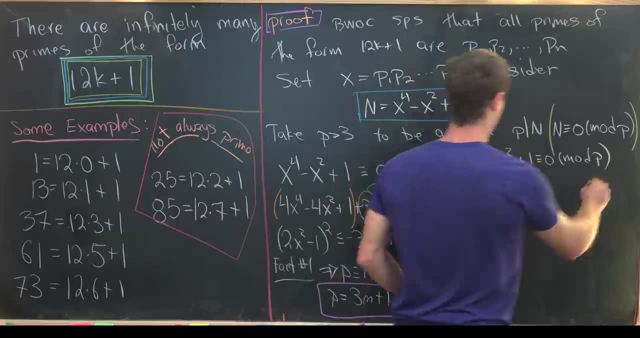 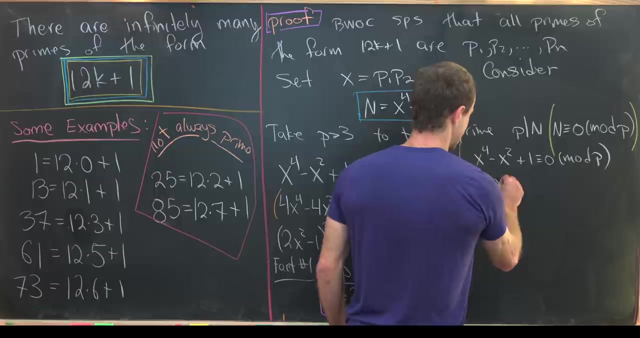 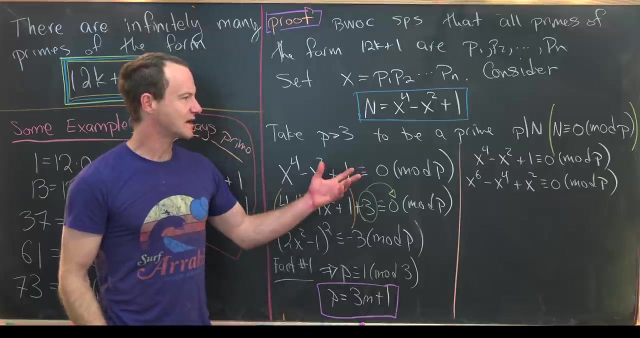 a similar version to it. so i'll take this: i'll have x to the fourth minus x, squared plus one, congruent to zero mod p. now i want to multiply that by x and see what we have. so we'll have x to the sixth minus x to the fourth plus x squared, congruent to zero modulo p. but now i can combine. 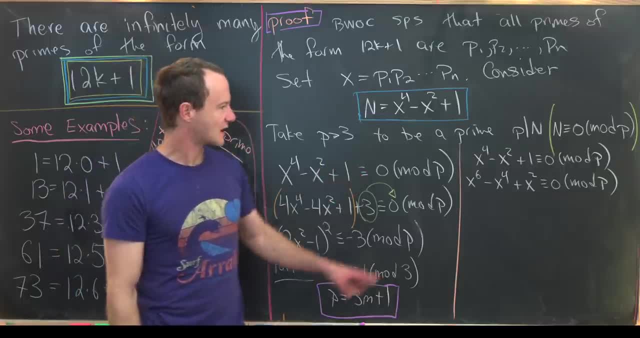 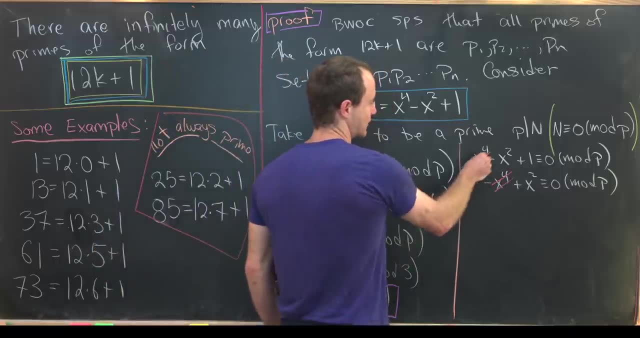 these and a bunch of stuff will cancel. in fact, what i want to do is add these two congruences. if i add these two congruences, this x to the fourth will cancel this x to the fourth, this x squared will cancel this x squared, and i'm left with x to the six plus one is congruent. 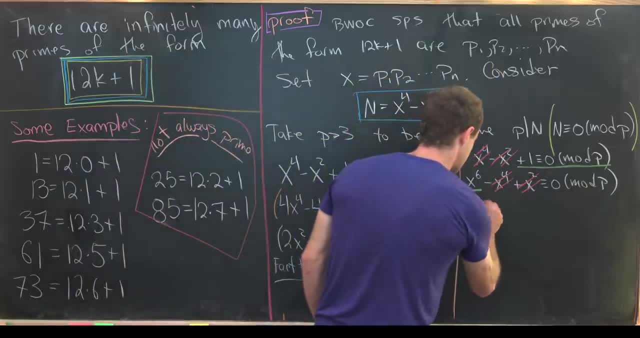 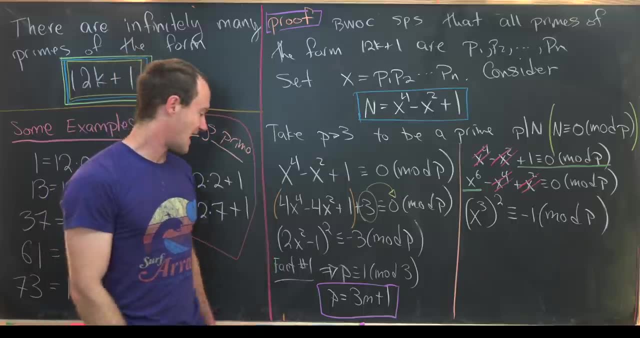 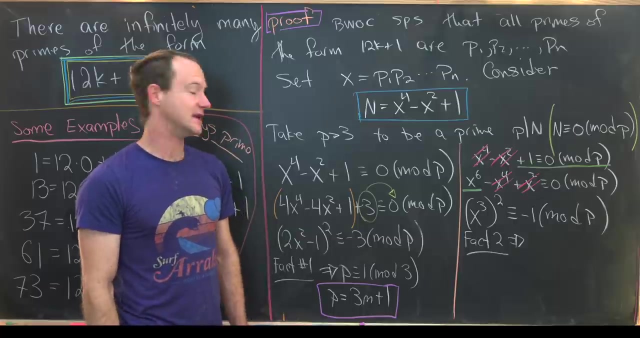 to zero modulo p, and i'm left with x to the sixth minus x to the fourth, plus x to the fourth, 0 mod p. In other words, x cubed squared is congruent to negative 1 modulo p, But by fact 2, that tells us exactly what form p is. So it doesn't really matter that this is x cubed. 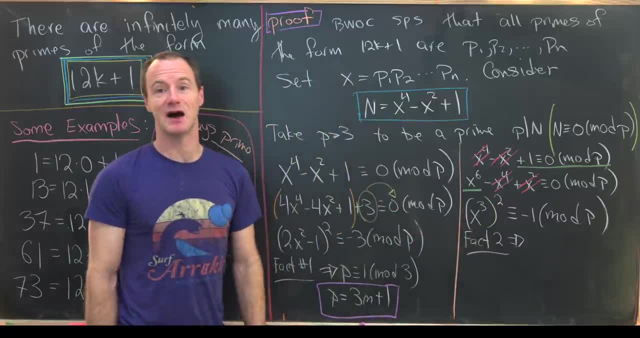 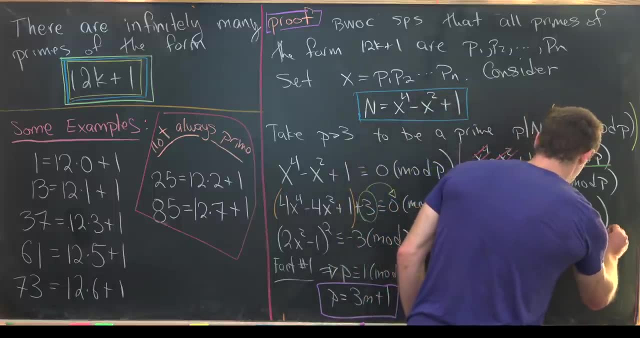 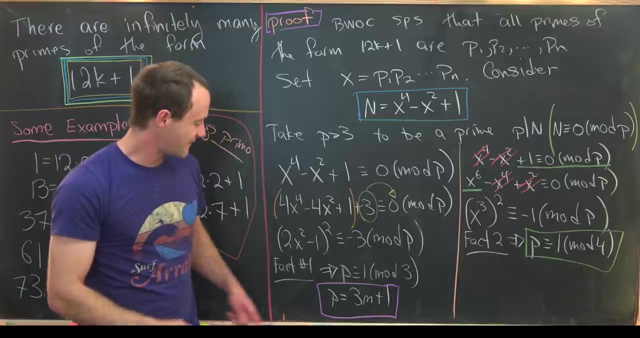 squared. All that matters is that we're squaring with something and getting minus 1 mod p. That tells us that p is congruent to 1 modulo 4.. Okay, so let's maybe put a green box around that, But now the fact that we have p is congruent to 1 mod 3 and 1 mod 4.. So in other words, 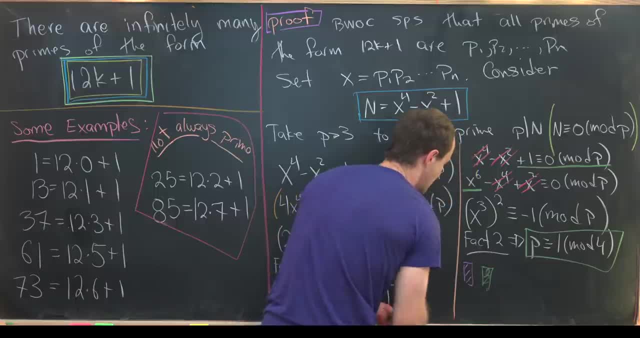 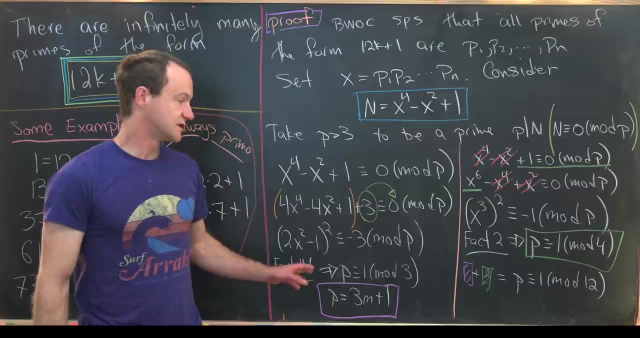 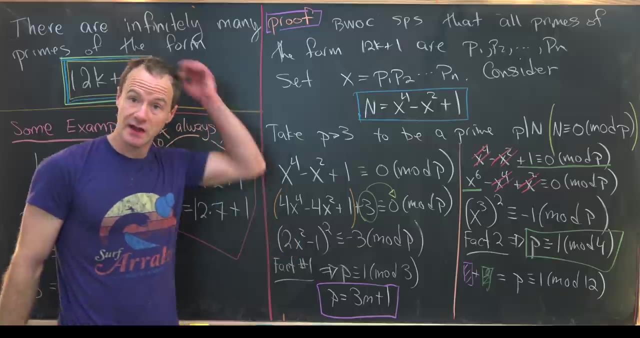 purple box plus green box means that p is congruent to 1 mod 12.. So having a remainder of 1 when dividing by 4 and simultaneously having a remainder of 1 when dividing by 3 means that you have a remainder of 1 when dividing by 12.. That's the kind of thing. 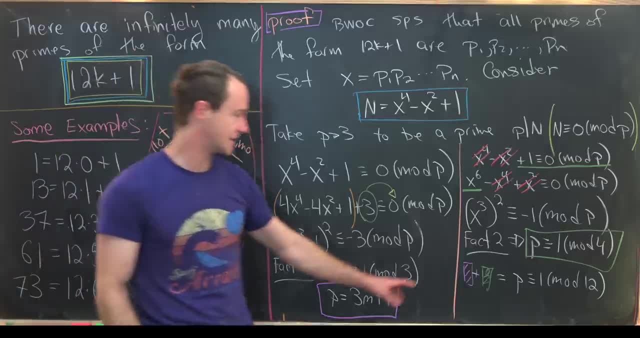 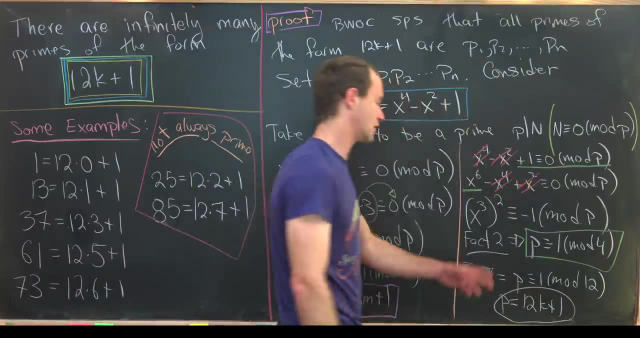 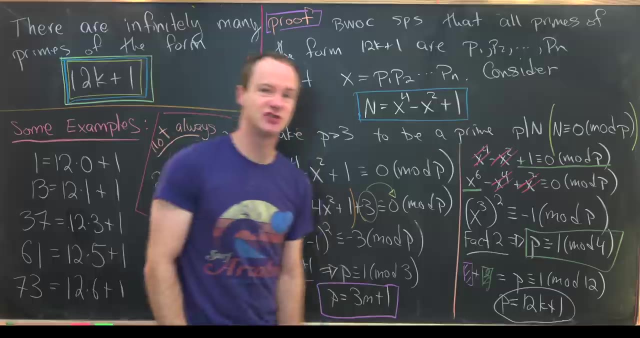 you do at the beginning of learning modular arithmetic. Okay, but that means that p is of the form 12k plus 1.. Again, that's an equivalent definition of being congruent to 1 mod p. Okay, so now let's take this fact which we've just taken, and we're going to take it to the 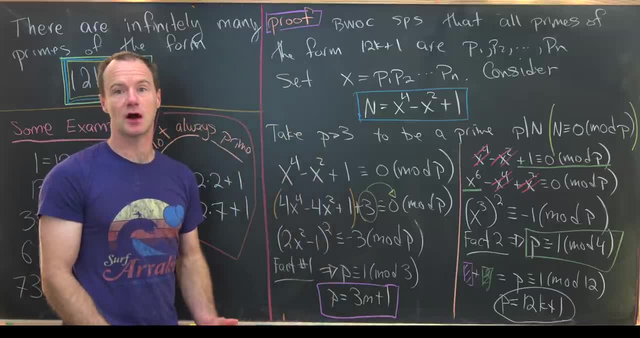 next step. We're going to take this fact which we've just derived, bring it up here, and then we can build our contradiction. So on the last board we found a prime p which was of the form 12k plus. 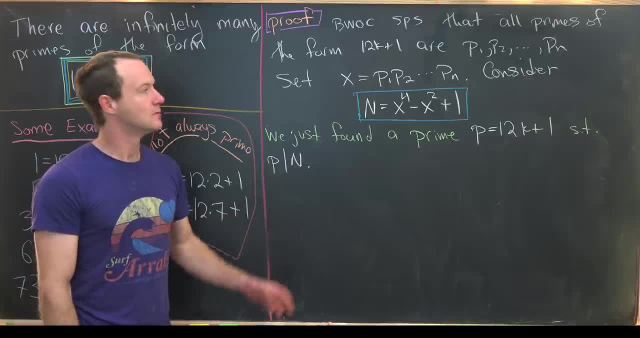 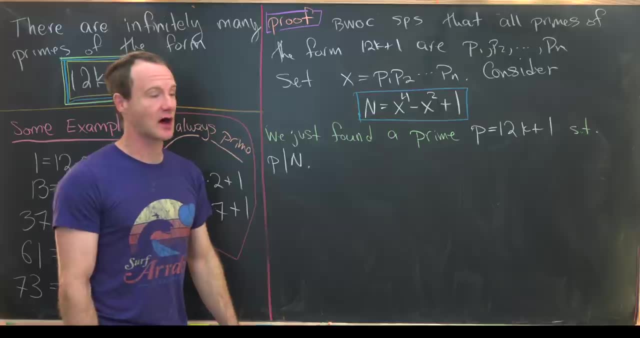 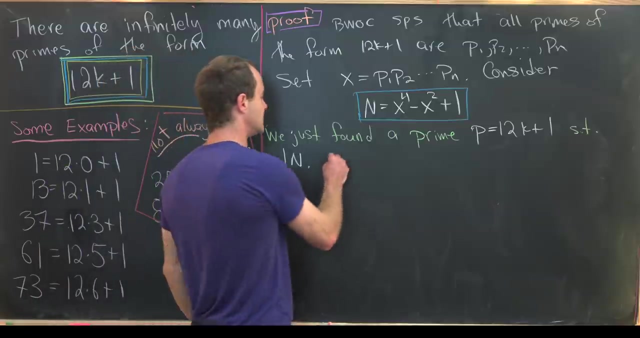 1 that divided n. But let's notice, by our assumption up here, which is towards the contradiction, we only have finitely many primes of the form 12k plus 1, and they're from this list, p1, p2, up to pn. So that means that the prime that we found 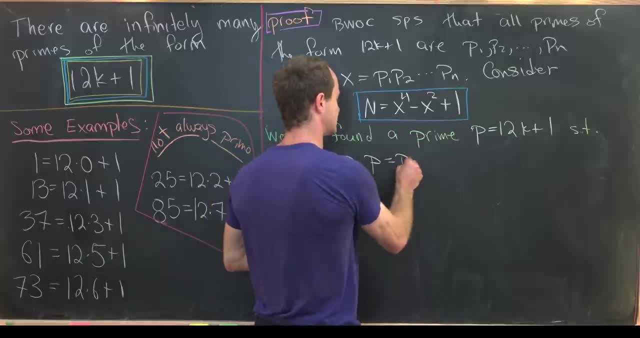 is of the form 12k plus 1.. So we can build our contradiction. So on the last board we found a must be on this list. In other words, we have: p is equal to pi for some i between 1 and n. 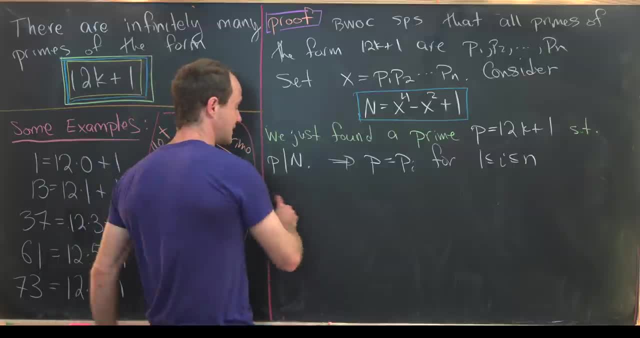 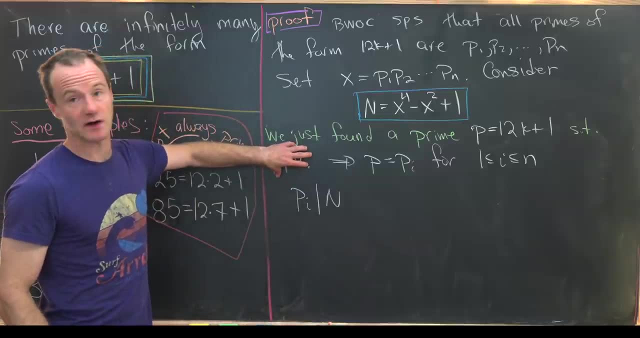 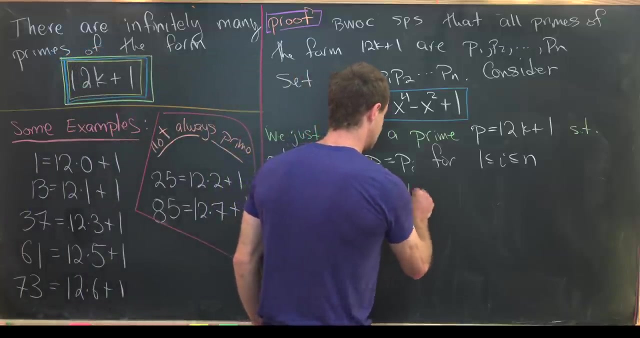 And that's going to cause quite a bit of a problem. Now that brings us to two observations. So pi divides n. That's just rewriting this fact right here, which is what we started with with p equals pi, And also pi divides x. Well, that's because x is a product of all. 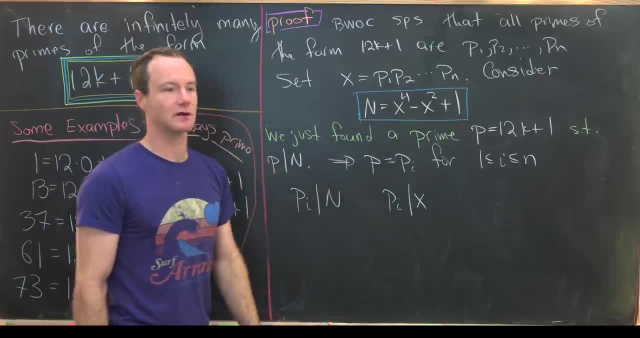 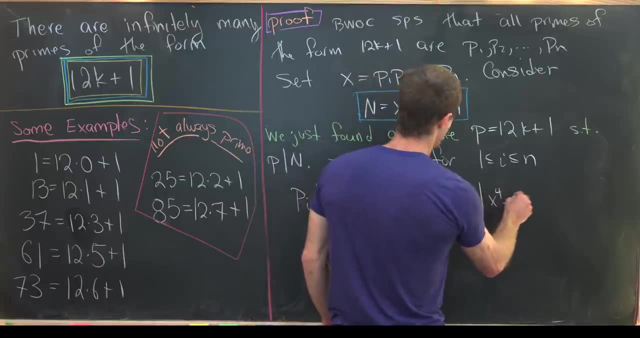 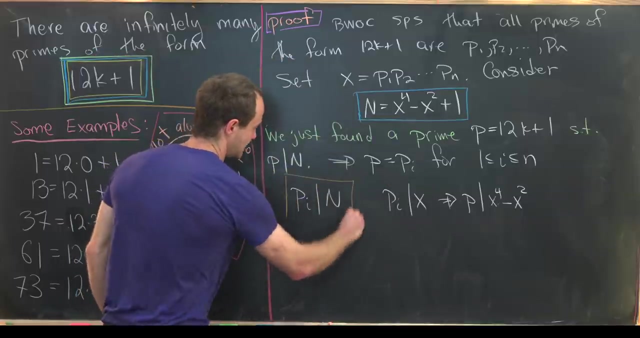 of these primes, including pi. pi is somewhere in the middle there. But if pi divides x, that means that pi most definitely divides x to the fourth minus x squared, because that's a multiple of x. But we're about to have a problem because if we put these two orange boxes together, 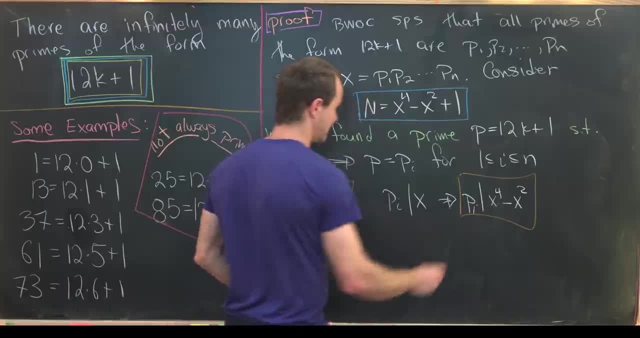 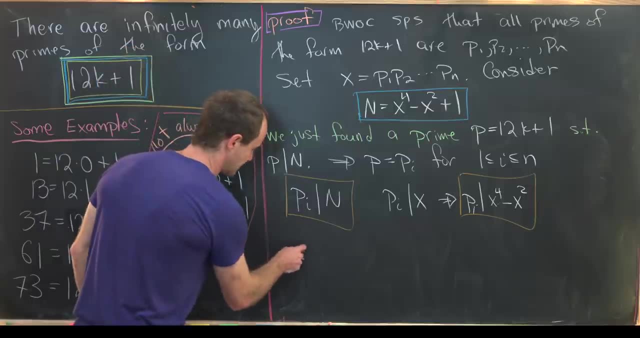 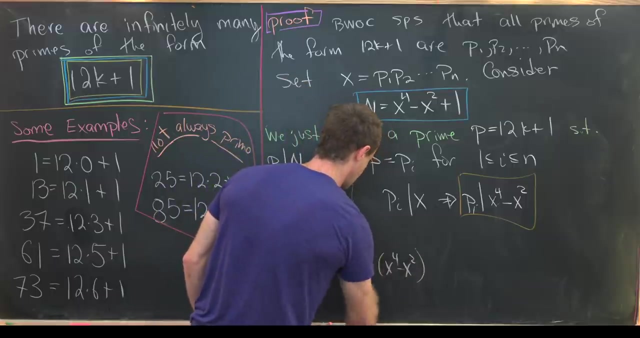 we can see that pi divides 1.. So if something divides a number and another number, it divides any linear combination. So if we put these two boxes together, we can see that pi divides 1.. of those two numbers. So in other words, we have: pi divides n minus x to the fourth minus x squared.